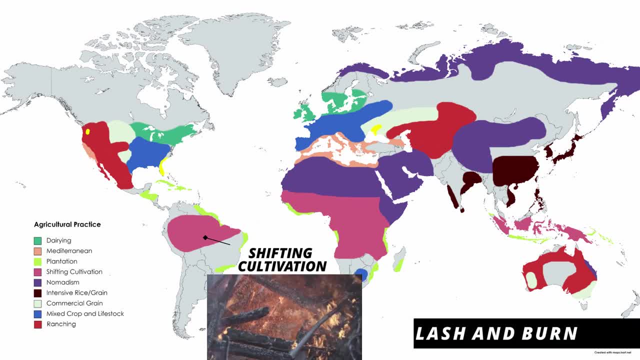 shifting cultivation is slash and burn agriculture- where you burn an area, cultivate, rinse and repeat, and generally seen in underdeveloped countries and not environmentally friendly in any way, shape or form. We also have ranching, which needs quite a bit of land. 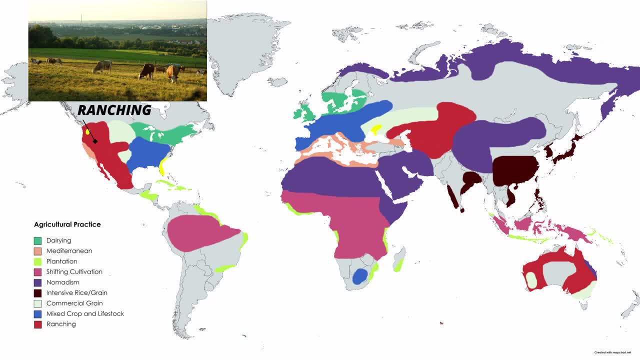 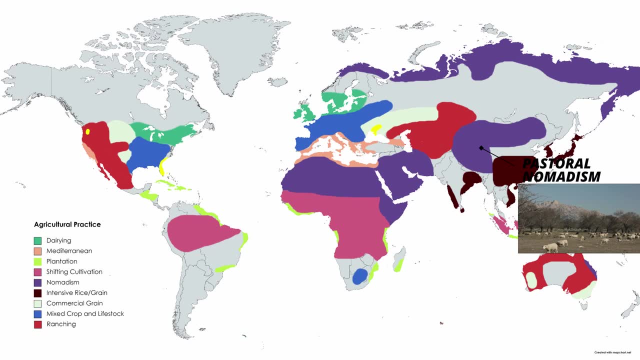 cattle need sufficient amount of space to roam about and you'll see ranching and dairying near each other, for obvious reasons, and they're mostly in cooler, more temperate regions. We also have pastoral nomadism, where they live a nomadic lifestyle and they're. 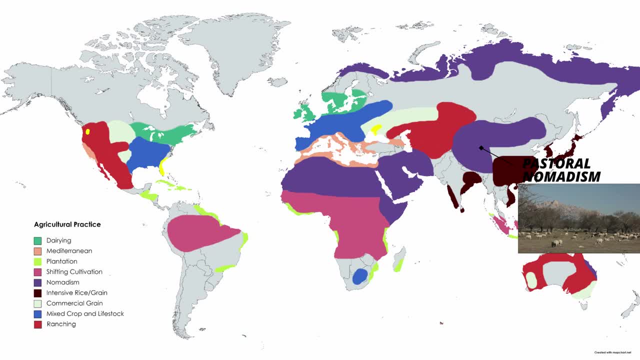 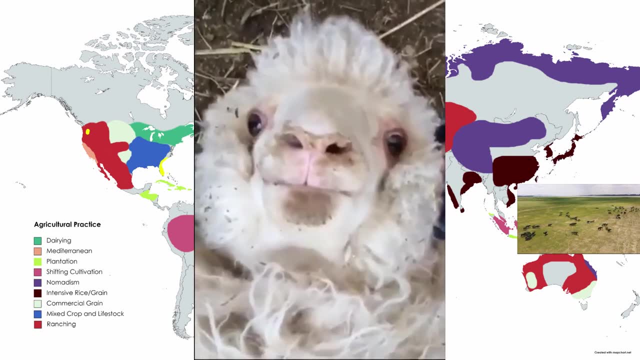 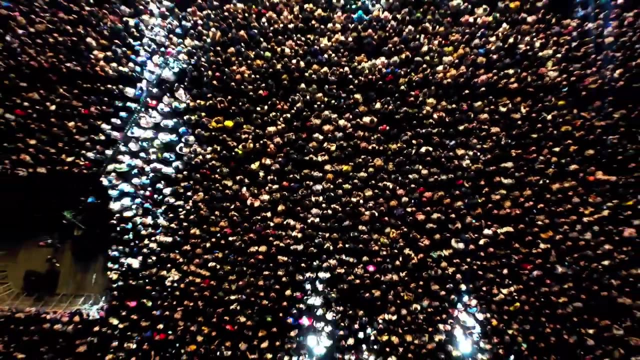 the most prevalent in uninhabitable areas like the Sahara or Siberia, And for the most part they're doing some sort of herding or traveling with goats, buffalo and sheep. The population increase that came along with the second agricultural and green revolution was accompanied with the globalization of 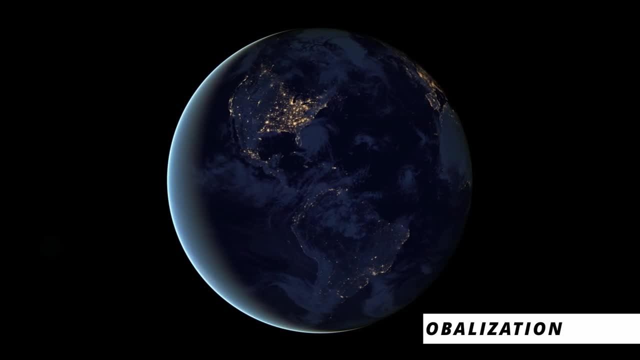 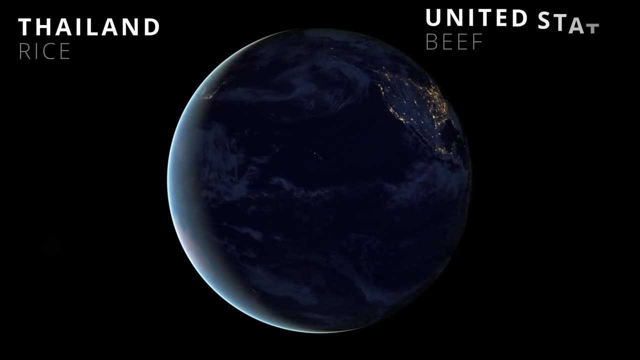 agricultural goods with countries specializing in their own respective products, thus establishing the global supply chain. For example, you have Thailand, who specializes in rice, exports US with their beef, obviously because of our unrelenting demand for Mickey D's Ecuador. 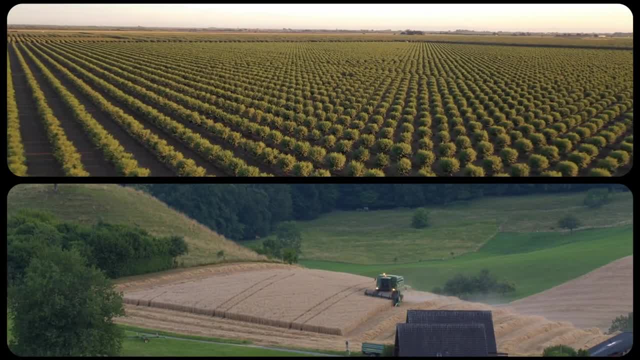 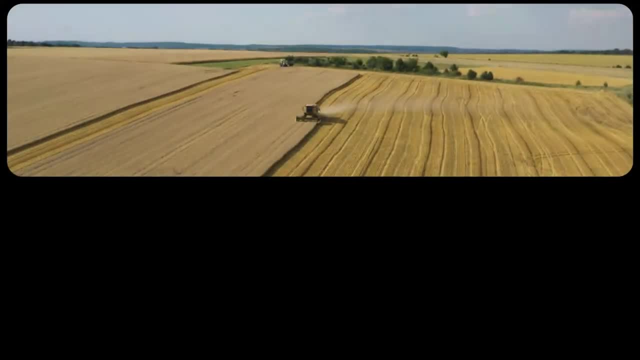 with bananas and Russian wheat. As the large scale commercial farms take over the smaller family farms, farming technology and tools- aka agribusiness- improves, So yields are going to increase in the land and we're going to see a lot of growth in agriculture. And 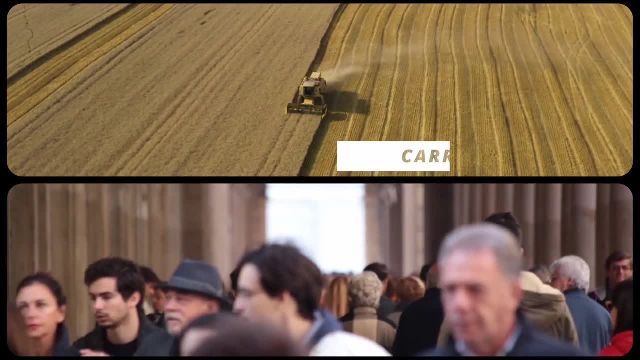 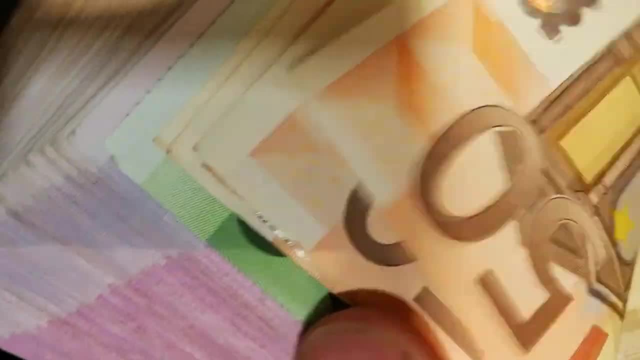 the land is able to support a larger population, thus increasing the carrying capacity of the land. This is also due to the fact that technology has also improved economies of scale, and I'm sure you all know what that is. but just in case your toddler sibling asks: let's go. 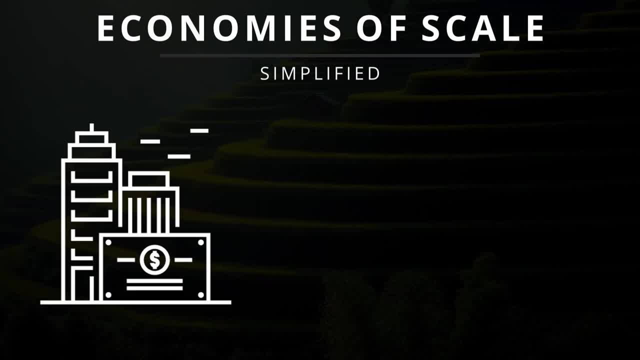 and break it down. Imagine there's a farming corporation and, with all their cash and investments, they decided to buy more tractors, pesticides and GMOs, which is going to increase their yields, and the cost of producing crops would be cheaper for the corporation, so they'll be able to make higher profits and ultimately, this allows the corporations to buy what they're after. So that's how they're going to be able to make higher profits and ultimately, this allows the corporations to support their farming, And I'm sure that if they do, they'll 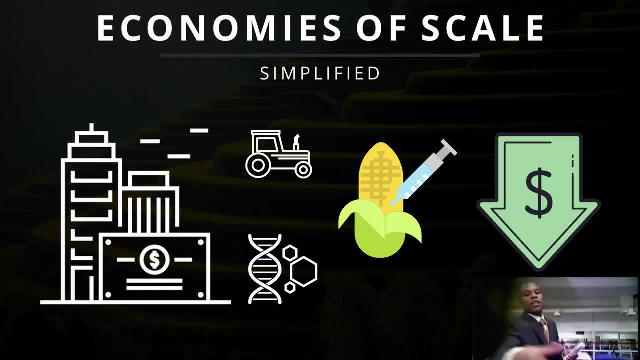 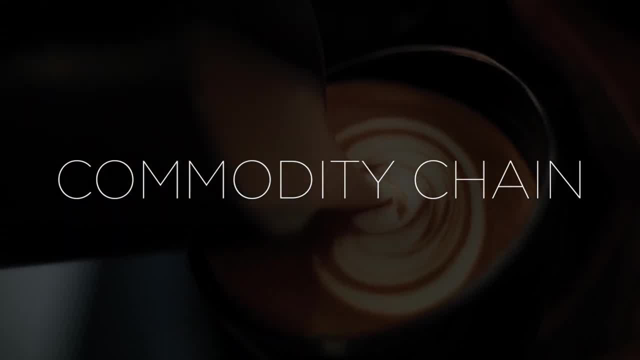 be able to make higher profits and ultimately this allows the corporations to grow. So I'm not going to to make you rain all day long. this increasingly globalized world is made up of commodity chains that connect the producer to the consumer, so let's use coffee as an example. you got the farmer. 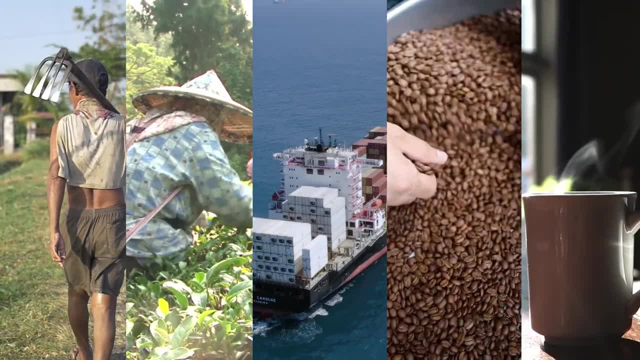 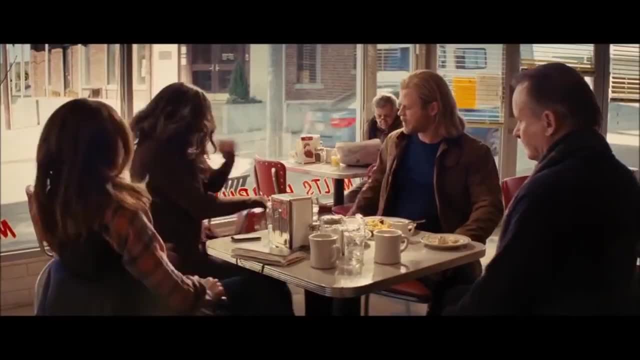 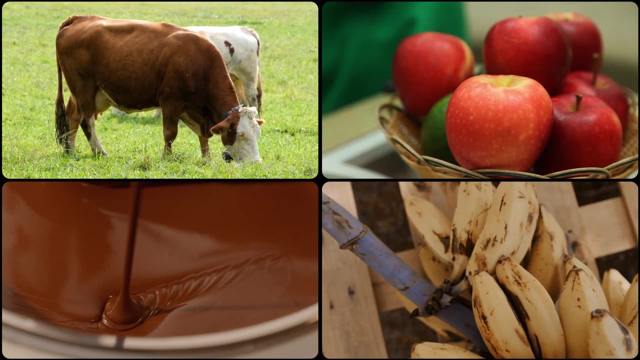 the extractor, the shipper, the distributor and then the final product. this drink, i like it, i know that's great. right another, i like it too, bud. so essentially, the commodity chain includes all the steps in between the producer and the consumer, and this process is seen in various goods around. 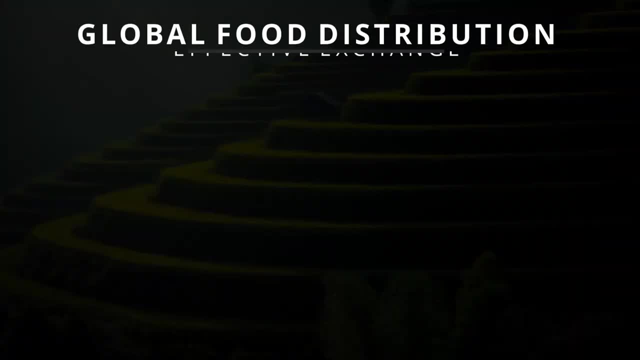 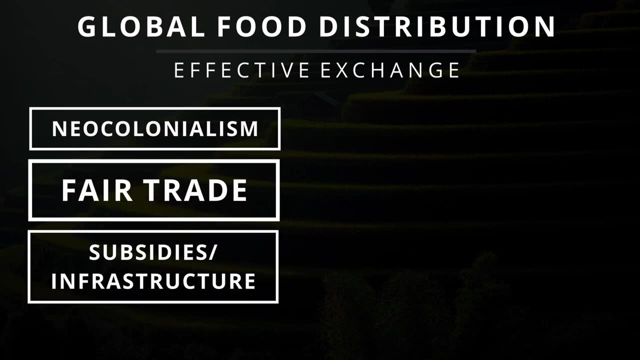 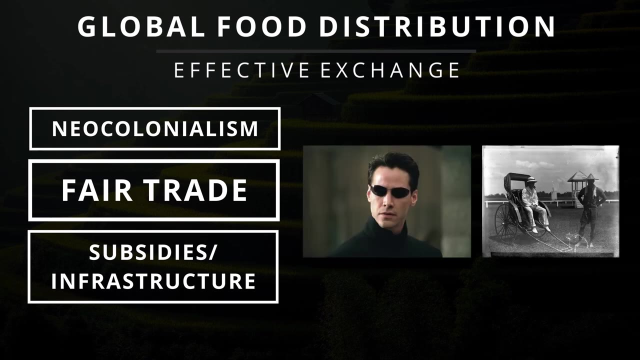 the world, like beef, apples, chocolates and bananas. there are a few things that contribute to the effective exchange of agricultural products around the world, and those include neo-colonialism, fair trade, subsidies and infrastructure. think of this as the so-called political side of food distribution. neo-colonialism represents a new form of colonialism that powerful countries are utilizing. 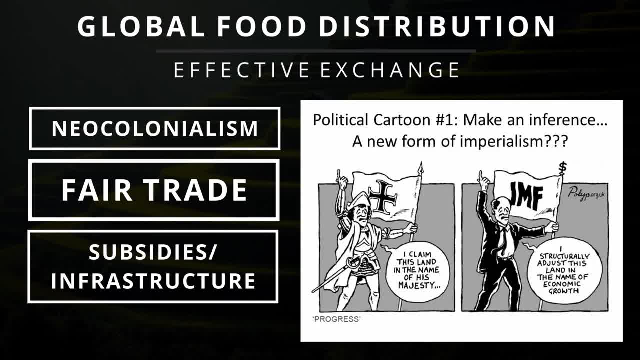 such as the us and china, and instead of completely dominating the countries, as they used to in the good old days, now they provide a false sense of political freedom, all the while maintaining relations for the sake of extracting money. then we have fair trade and think of this as a contract between: 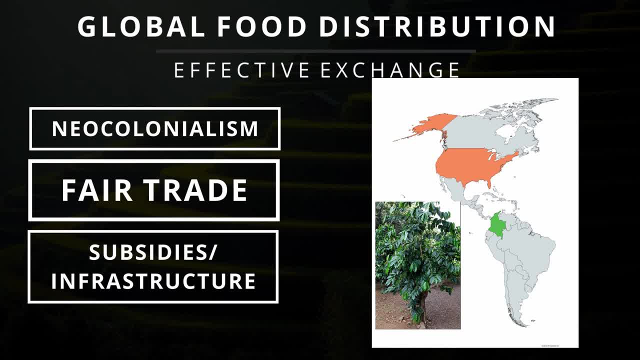 underdeveloped countries and the developed countries, so that the farmers in the underdeveloped countries have a chance at competing with the big boys. the farmers are also guaranteed certain prices, so that ensures the farmers in the third world countries are not being taken advantage of. lastly, for this section, we have subsidies and infrastructure, which are both things that are. 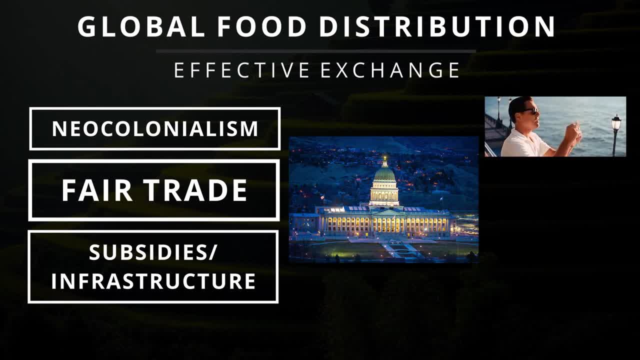 taken care of by the government. think of subsidies, as fuck the government gives to the farmers so that it guarantees certain prices, which incentivizes farmers to produce and to maintain a level of supply. infrastructure such as roads and ports are often built by the government, and this supports the flow of agricultural goods, not. 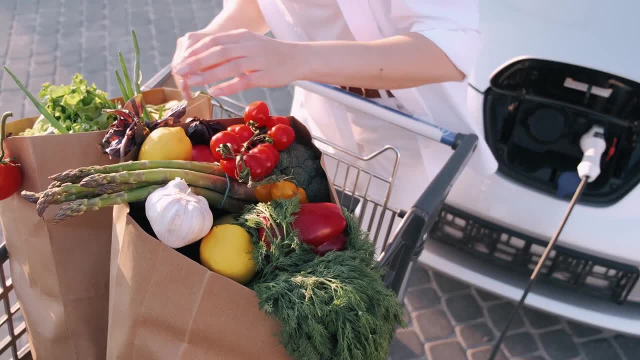 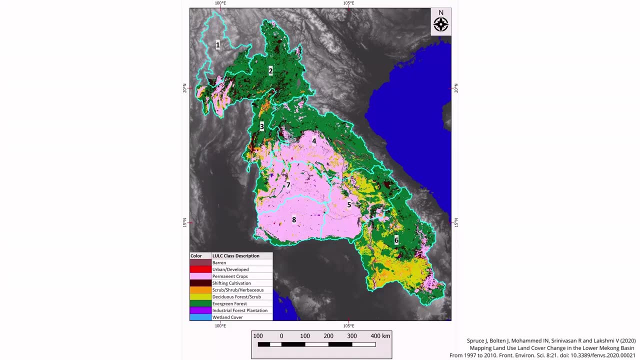 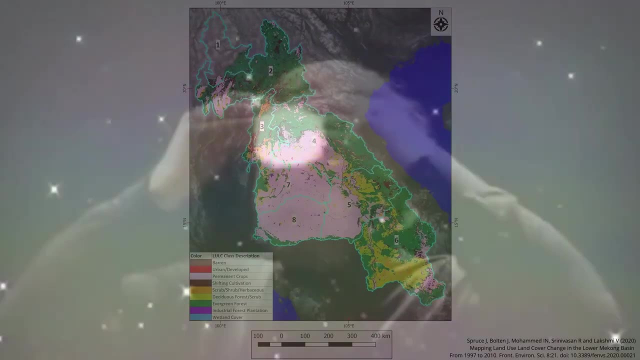 only in that country, but around the world. but all this talk about increased production ain't all sunshine and roses, and there are some consequences that accompany it. for example, we have land cover change, which means the type of land that covers the area has changed mind-blowing. i know you could see this in the mekong basin, which is in southeast asia. 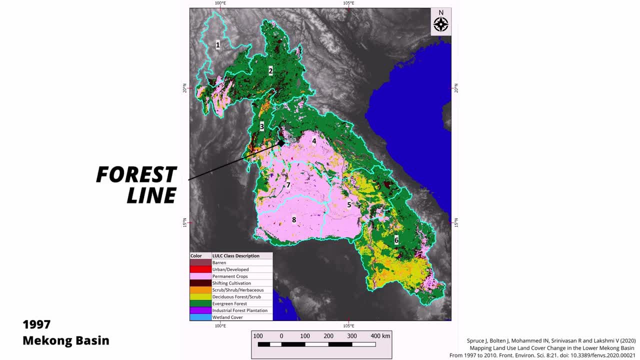 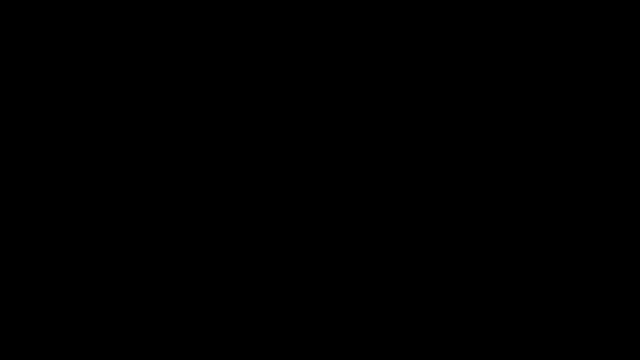 and notice the tree line in 1997 which is where the green and pink meet, and look how far back it receded in 2010, thus demonstrating that the land cover has changed. so then we got to dive into the environmental effects of all this farming and irrigation, and these practices can lead to. 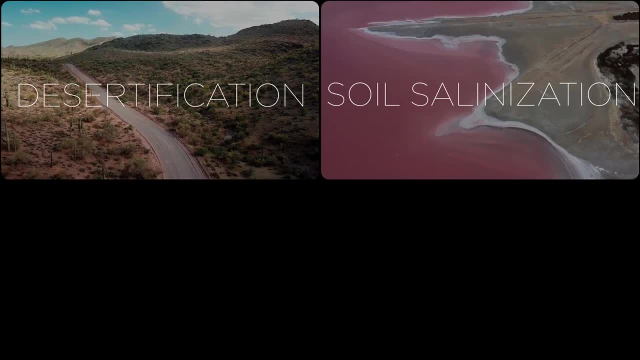 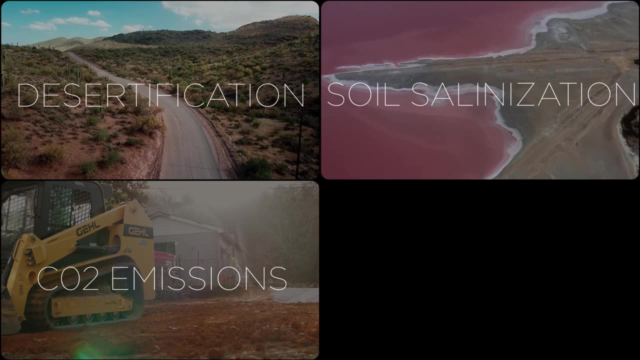 desertification where the soil is no longer fertile. soil salinization where the salt covers the land can happen due to improper irrigation practices. increase CO2 emissions as a result of the tractors and the draining of wetlands for the sake of making space for farmland, which ruins ecosystems. 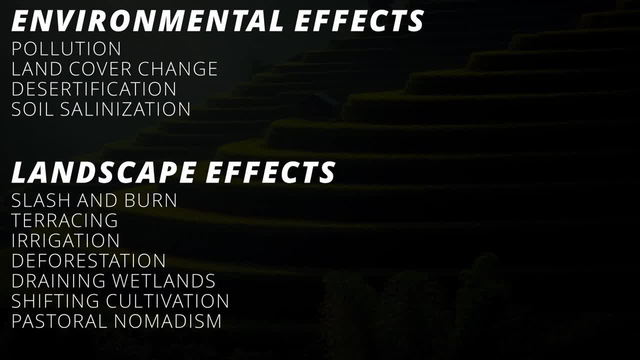 So here's a list of all the environmental effects, in case you want to pause and jot them down. and just a little hint for the FRQs: Teachers and AP graders love it when you use terms like ecosystem, flora and fauna, which just means plants and animals. the ozone layer. 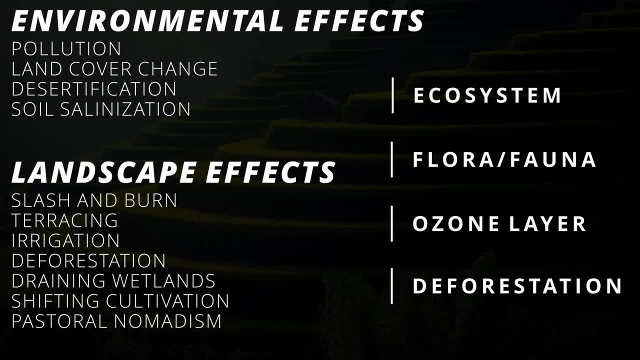 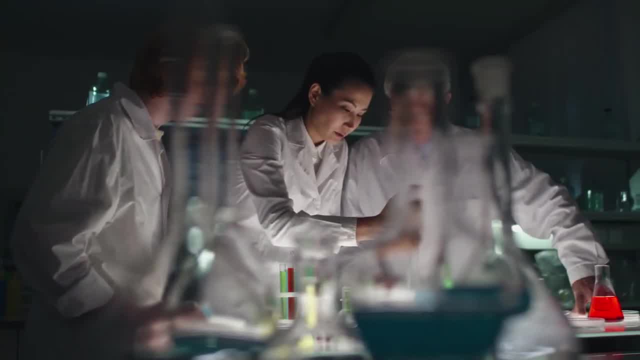 and deforestation, instead of saying it affected the environment. These phrases make the graders think: nice, this person actually knows what they're talking about. Even though we have all this new agricultural technology around the world, people sometimes wonder why we have hunger in some. 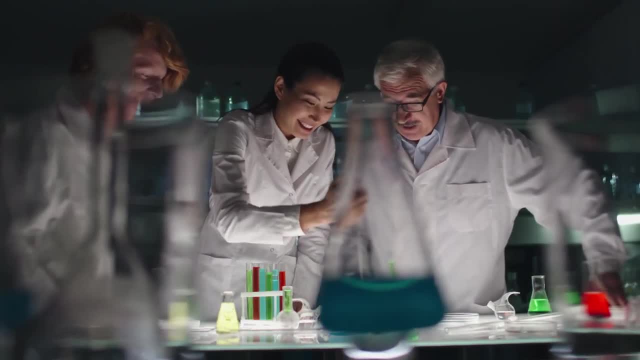 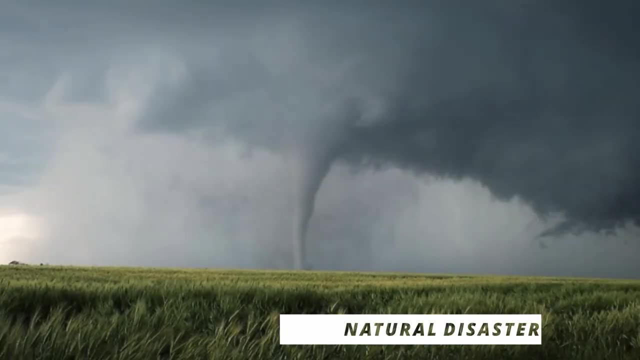 countries, and this is due to the challenges that we face. For example, distribution is a huge problem, as we're not sure how to export food to the poorer countries before it rots. Natural disasters can lead to a loss of harvest or livestock. Suburban sprawl. 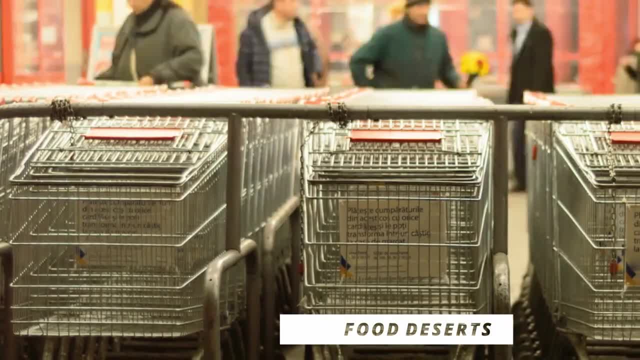 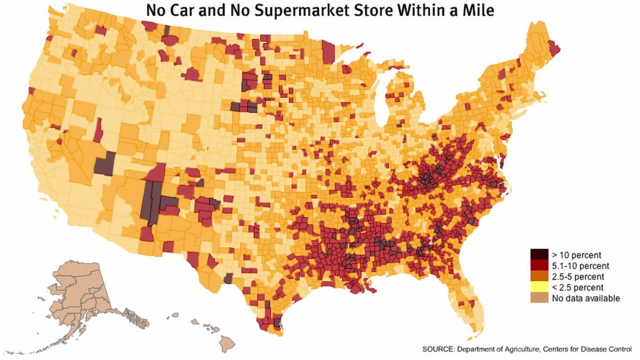 taking up more and more farmland. And, lastly, food deserts exist in certain parts of the US, which means that grocery stores are not setting up shop in the poorer regions, and this can lead to a lack of access to fresh foods and malnutrition. 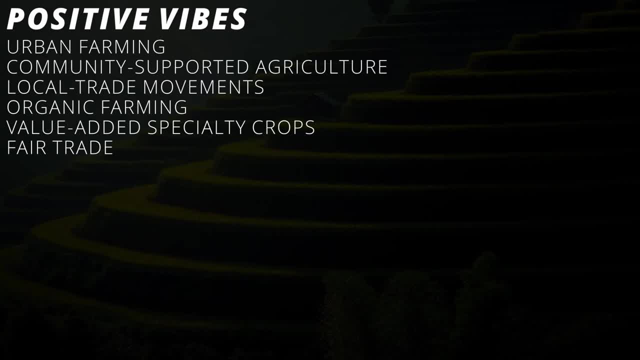 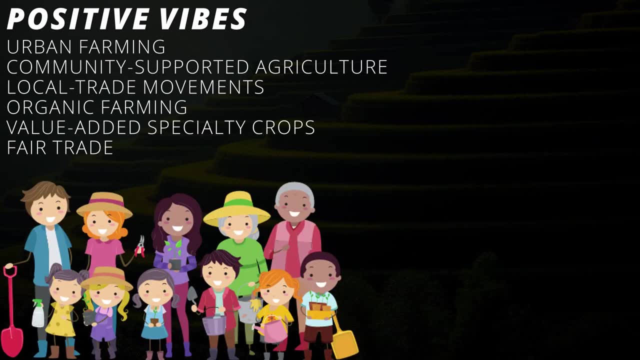 However, it's not all negative up in the agricultural realm and we do have some positives, starting with urban farming, which grants access to fresh foods in metropolitan areas, Community-supported agriculture, which guarantees that a community will support a farmer by buying their crops. And, finally, food deserts exist in certain parts of the US. 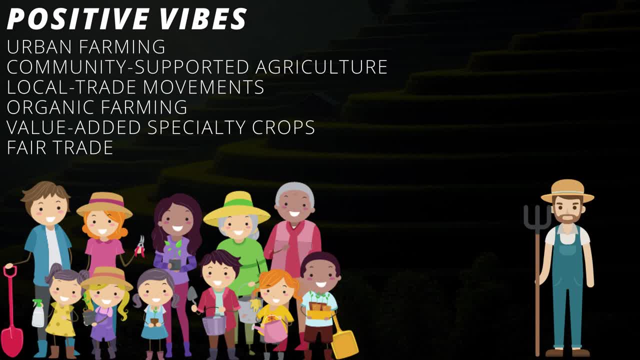 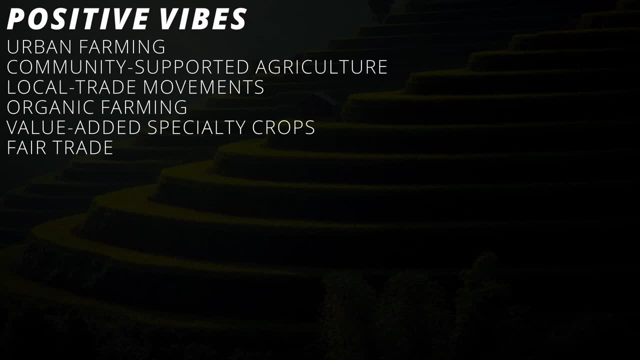 which means that a community will support a farmer by buying their crops. Think of it as a Netflix subscription service, but with farming, and the effects are that it gives the farmers more money so that they can make you. We're not doing that again. Then we have the value-added specialty. 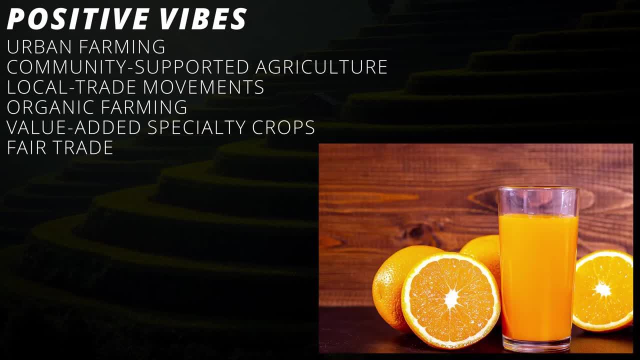 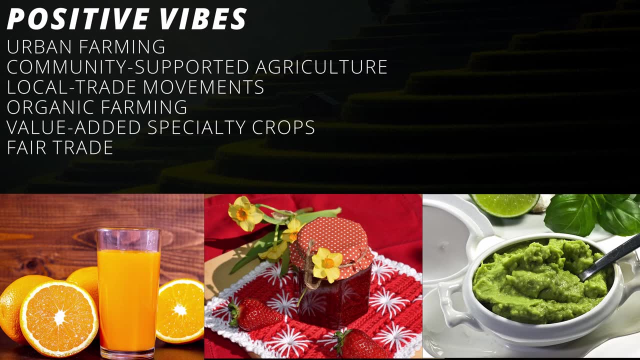 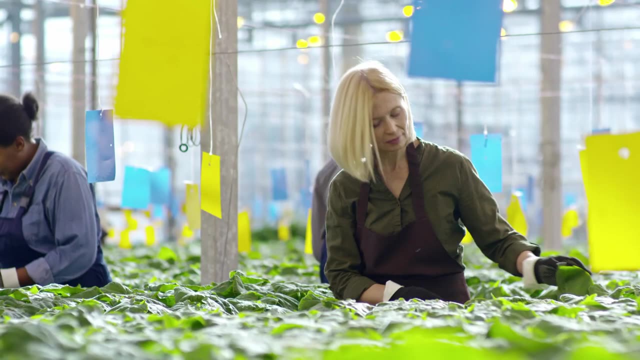 crops- and I want you to finish the phrases: Orange, strawberry, waka and all those are examples of value-added specialty crops, because it allows the farmers to charge more for processing the crops, thus giving them more money so that they can make you. Last but not least,